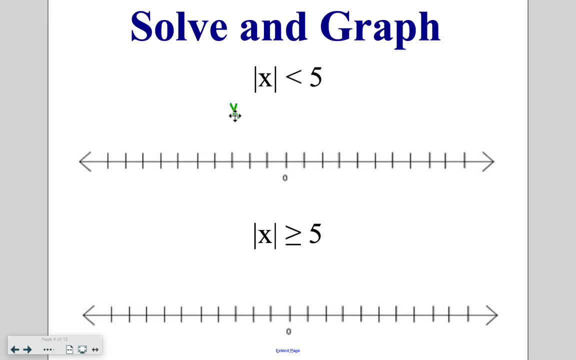 than five. I'm going to start with the absolute value of five. I'm going to start with the absolute value of five. The first statement here is going to say x is less than five. So if I put that on the graph, I would go over one, two, three, four, five open circle and moving to the left, because we want it. 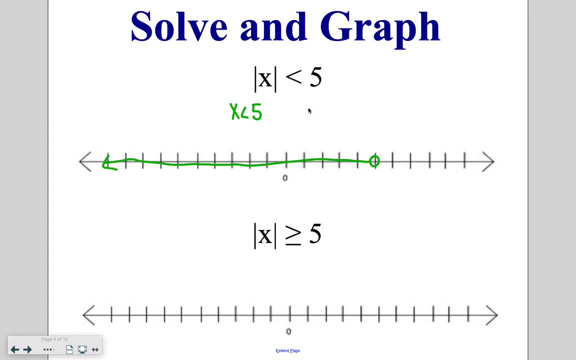 to be the values that are smaller. Then I'm for case two. I would say x, flip the inequality sign to a greater than and then change it to negative five. Now this would go over to negative one, two, three, four, five, and then it's getting bigger now. So this is once again one of those and cases where 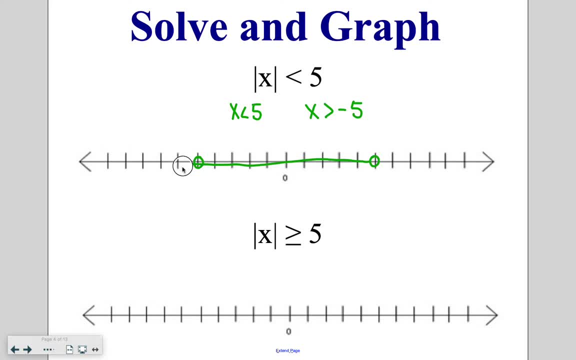 it's between those values. So you can see on the graph when we have the less than it's going to end up between those two numbers that we have. Moving on to the greater than case, If I have my first statement, it's going to be: x is greater than or equal to five. So I go over to one, two, three, four. 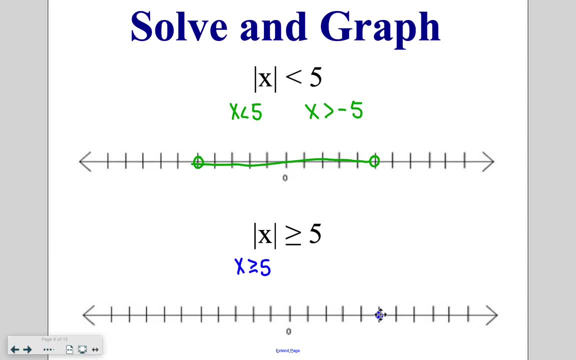 five. In this case it's a filled in dot and then it says greater than. So that is moving to the right. With case two, then it's still x, Flip that inequality sign to less than and change it to a negative five. So I go negative one, two, three, four and five. Put once again my filled in dot, my closed. 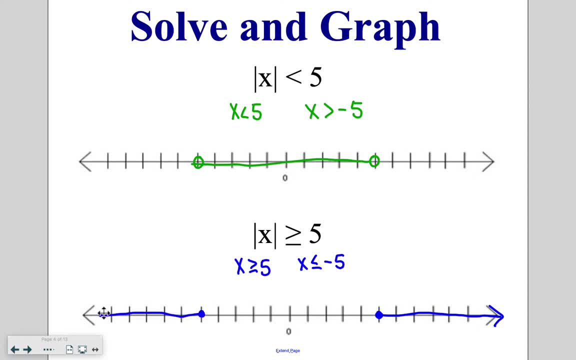 dot and then these ones are moving to the left. So you can see that this greater than statement is going to give me the or case where they are moving outside of that given range. So the less than or less than or equal to this is the and scenario where it's between the greater than or. 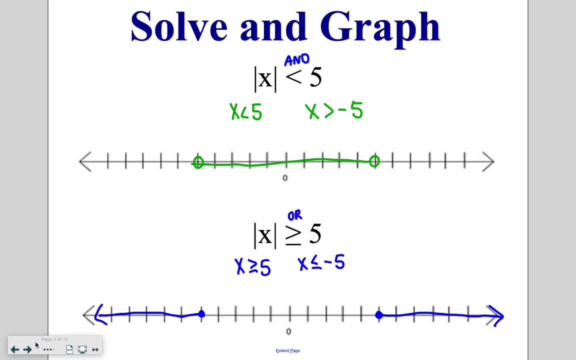 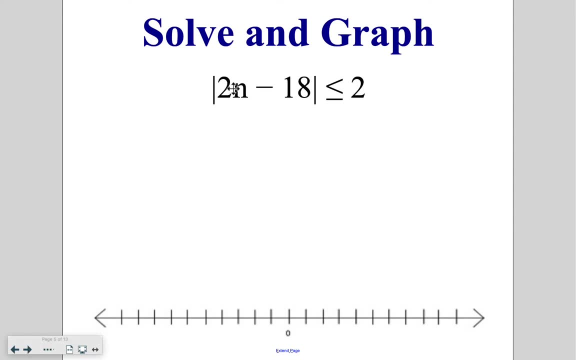 the greater than or equal to are the or scenario. Now we're going to do a couple examples where we have a little bit more complex problem. So I've got the absolute value of 2n minus 18 is less than two. First thing we want to identify is that this is less than or equal to, So it's going to be an. 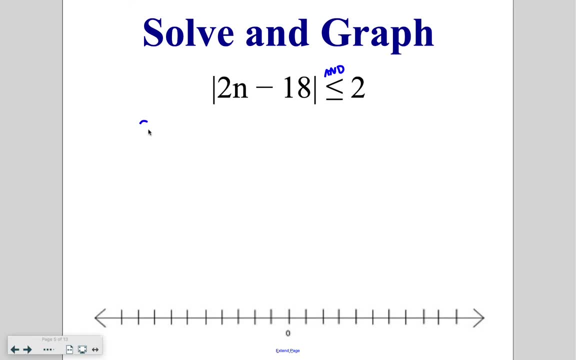 and statement, Then I'm going to break it into case one and case two. So 2n minus 18 is less than two is going to be case one, And then the same part, 2n minus 18 is greater than or equal to. 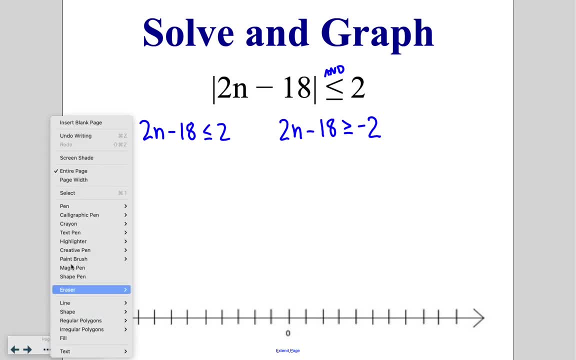 negative two for that second case, Then we're going to go ahead and solve both. So the first thing we're going to do is add in the negative two. So we're going to go ahead and solve both. 18 to both sides and that's going to give me 2n is less than or equal to 20.. And dividing by two on 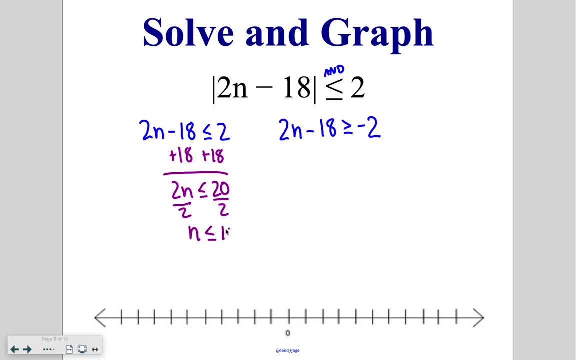 both sides I get n- is less than or equal to 10.. When I come over and solve the one on the right- so this case two, once again I'm going to add 18 to both sides and that's going to give me 2n is. 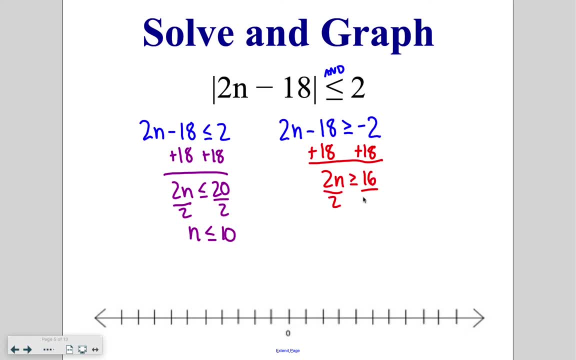 greater than or equal to 16.. Dividing by two on both sides I get: n is greater than or equal to 8.. So my statement now says n is less than or equal to 10 and n is greater than or equal to 8.. So if you write that as one compound inequality, it's 8 is less than or equal to n. 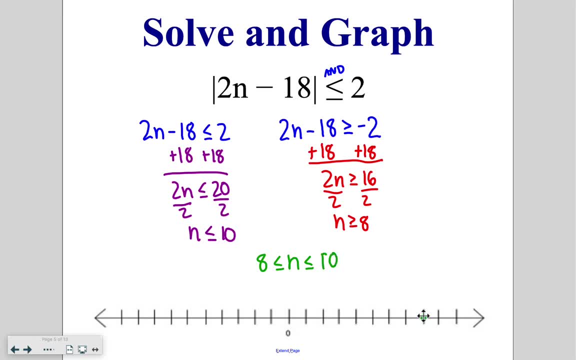 which is less than or equal to 10.. So I'm going to put my two dots on my graph. and because it is an and statement, those answers are in between. An example of an or statement: We've got a greater than, so we know that it's or. Once again, we take it and break it down into case. 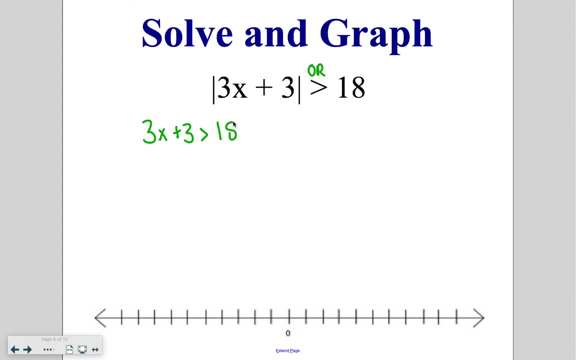 one, which in this case, is 3x plus 3, is greater than 18, or case two, which is 3x plus 3, is less than negative 18.. Once again, we are going to start by solving case one, subtracting 3 on both sides. 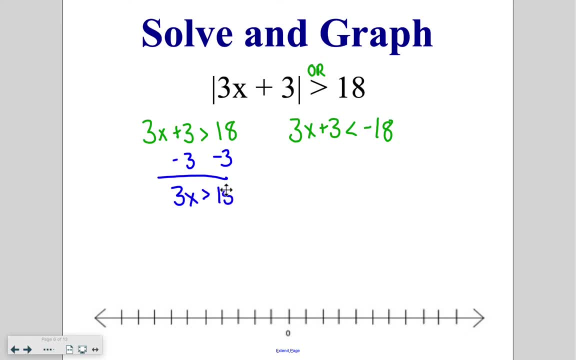 gives me 3x is greater than 15.. Dividing by 3 on both sides of that inequality- I end up with x is greater than 5.. When I move on to solve case two, once again start by subtracting 3 on both sides, so I have 3x is less than negative 21.. Dividing by 3 on both sides of the inequality, 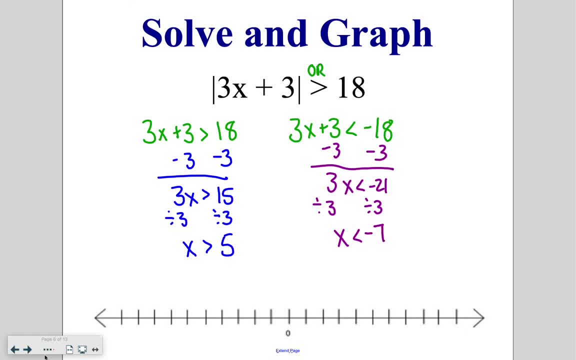 gives me x is less than negative 7.. So now my final answer says x is greater than 5 or x is less than negative 7.. So, because it's an or statement, we have the two separate pieces to graph. First we go over 1,, 2,, 3,, 4, 5. Open dot and it is getting bigger, so it is moving to the right, And then with 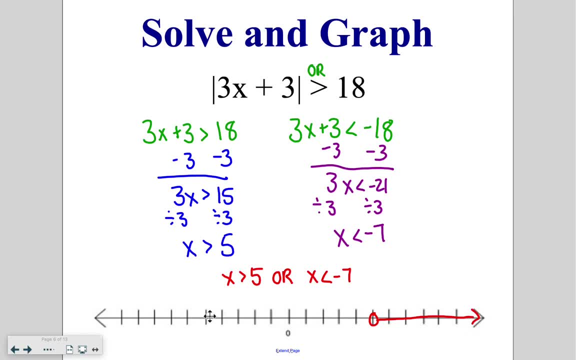 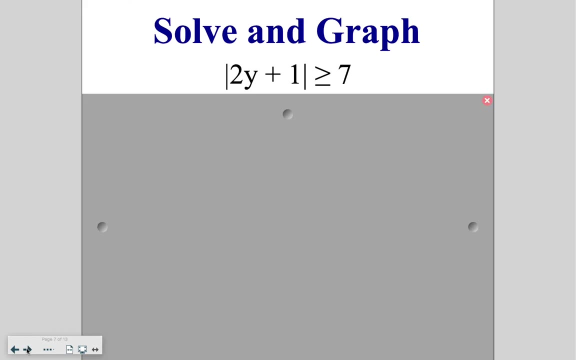 your second one negative: 1,, 2,, 3,, 4,, 5,, 6, and 7.. Once again, open dot. It is less than so. we are moving to the left. Go ahead and try this one On your own. First, I want you to tell me: is it an and or an or statement? It's an or statement because I have 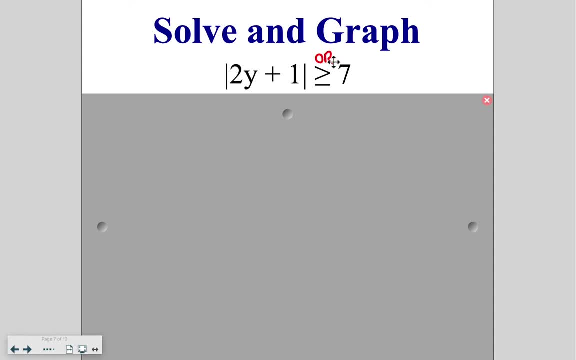 greater than as my inequality sign. Go ahead and solve case one and case two. When you solve case one and case two, I've got y is greater than 3 or y is less than or equal to negative 4.. Now I want you to tell me the dot and the. 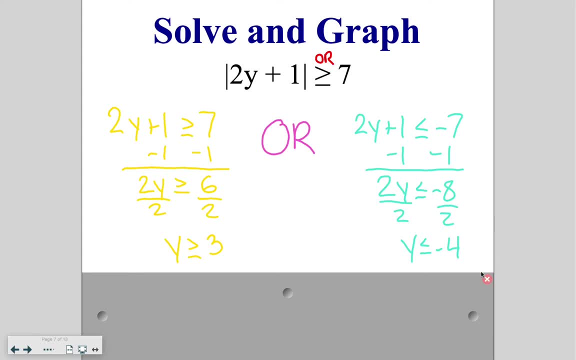 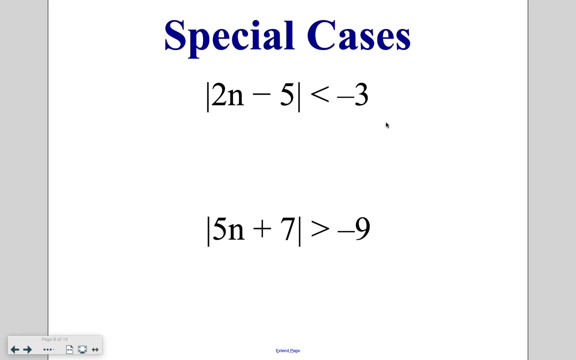 direction for both of these inequalities. For case one, it is a closed dot moving to the right. For case two, it is a closed dot moving to the left. There are a couple special scenarios when we have these absolute value inequality statements. Remember, absolute values are always positive, So what this first one is saying is a positive value is. less than a negative value. So if we set h for x and a 0 in order to return the soldier value which is greater than 2 for the just 1 for x, then the water times h will seeae much. and then I will see here evenethrough the last quarter: in total the total of E is less than 7 in the total times L. 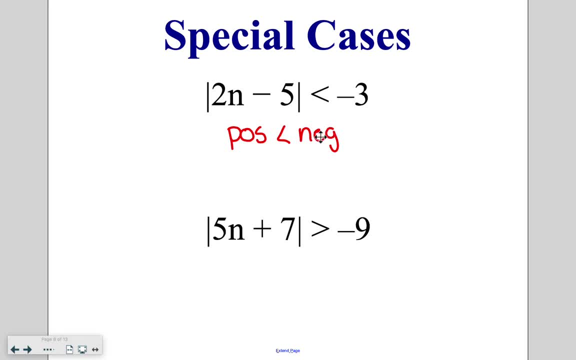 value. We all know that positives are not less than negatives. So if you ever see a statement that says an absolute value is less than or less than or equal to a negative, this is going to be a no solutions scenario. So if it's less than, it is a no solution problem. If we flip down to the 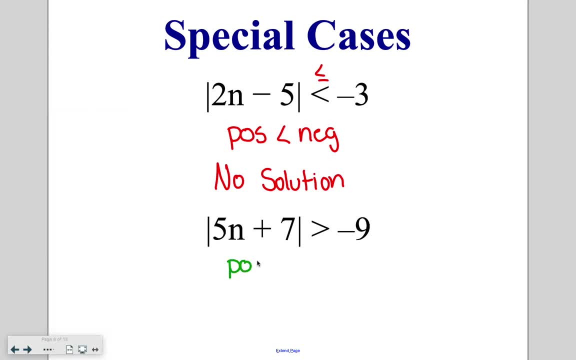 other case, where it's greater than, this says a positive value is greater than a negative value. We know that all positives are bigger than all negatives, So if it is greater than, or greater than or equal to, with an absolute value compared to a negative, this is going to be the all solutions. 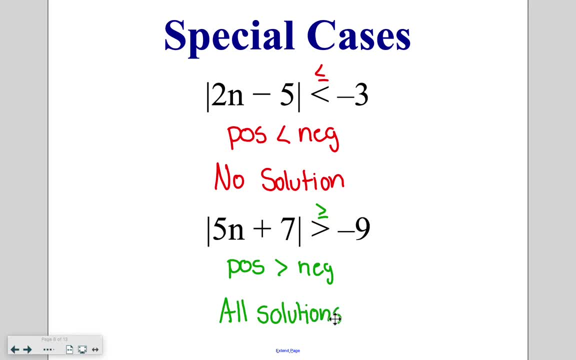 scenario, Any number you plug in is going to work. So, once again, if it's comparing the absolute value to a negative, it's going to be a no solution problem. So if it's greater than or equal to a negative number, it's either going to be no solutions in the less than, less than or equal to. 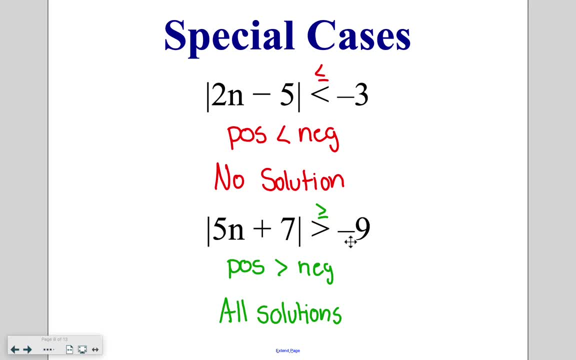 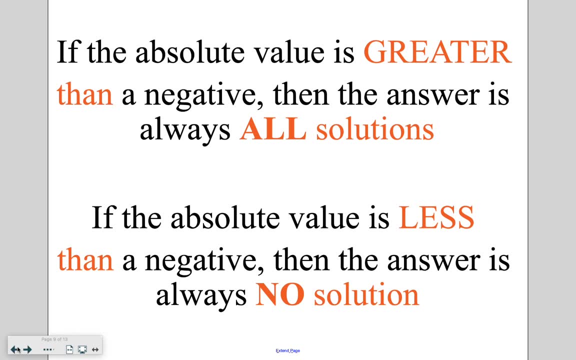 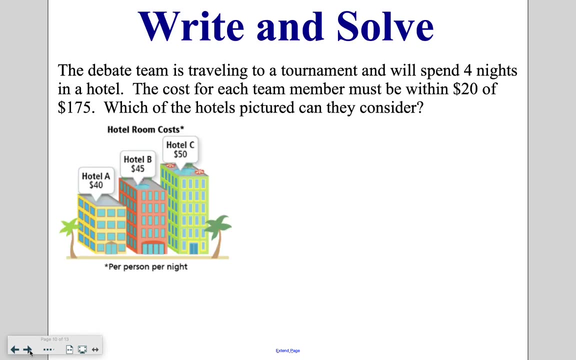 case or all solutions in the greater than, or greater than or equal to case. So here's just one more time that recap: If it's greater than it, is all solutions. If it is less than it, is no solutions. Word problem: here We've got a debate team is traveling to a tournament and 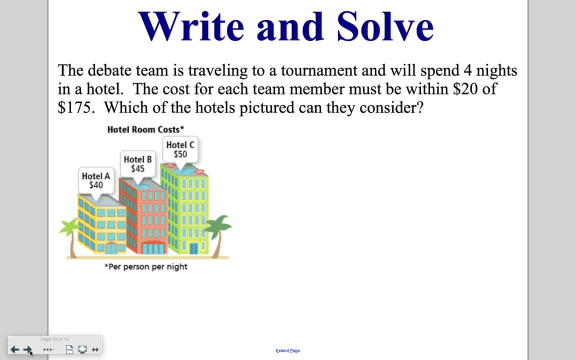 will spend four nights in a hotel. The cost of each team member must be within a year. Our total cost of each team member is $1.20 of $1.75.. Which of the hotels pictured can they consider? So our first job is to write out the inequality statement. If you remember from chapter 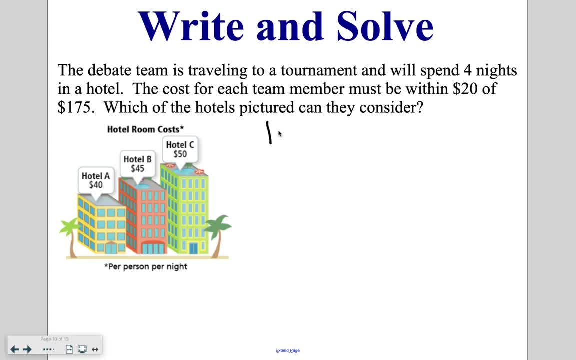 two, our inequality or, excuse me, our absolute value statements have a general formula of x minus the average or the middle value, And then it used to be equal. Now we're going to have to decide if it's greater than or equal to. So we're going to have to decide if it's greater than or. 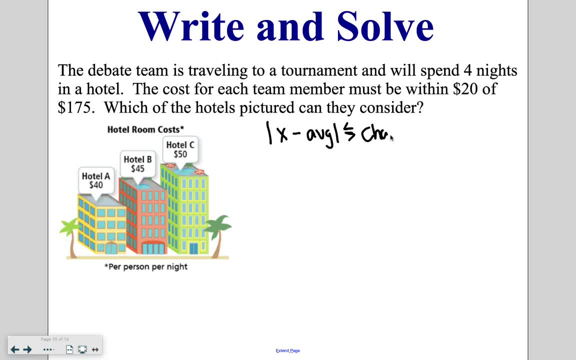 or less than, and then the amount that we can change by. So in this case, the first thing it tells us is that they're spending four nights. So if they're spending four nights, that's gonna be four Xs- The average, the middle amount that they want to spend. 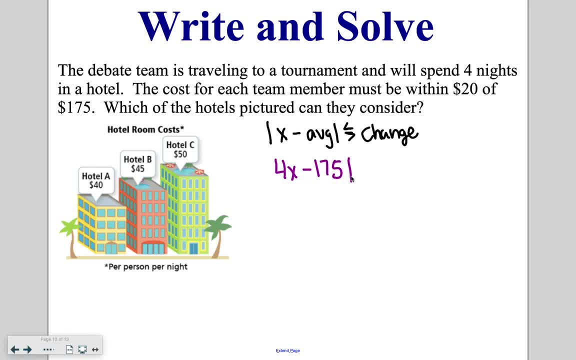 is $175. So inside my absolute value bars I've got four X minus 175.. Because it says within, that's a synonym of between, So that means it's going to be less than or equal to in and case 20.. 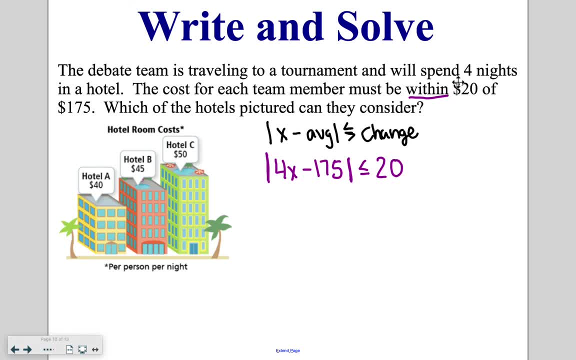 We include the equal to, because it could be $20.. The answers could be $20.. So now that we've written our inequality, we're gonna go ahead and split it into case one and case two. So four X minus 175 is less than $20. 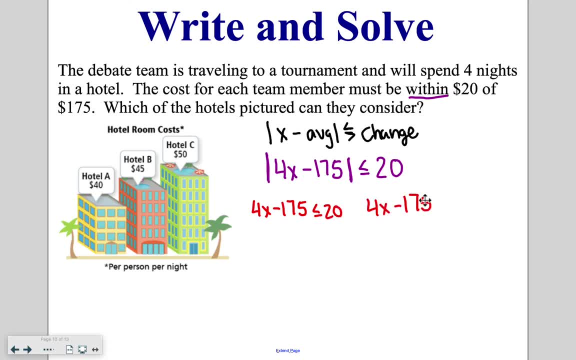 And four X minus 175 is greater than or equal to negative $20.. Solving case one, I'm going to add 175 to both sides of the inequality, which is going to give me four X is less than or equal to $195. 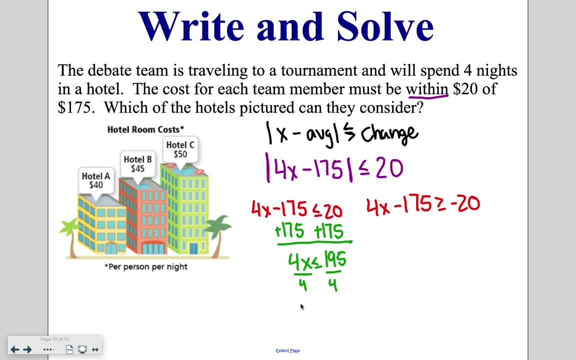 Dividing by four on both sides gives me that X is less than or equal to $48.75.. If I go through and solve case two, I add 175 to both sides, And when I do that I get four. X is greater than or equal to $155. 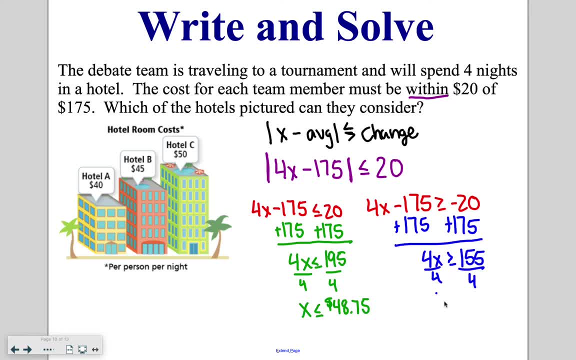 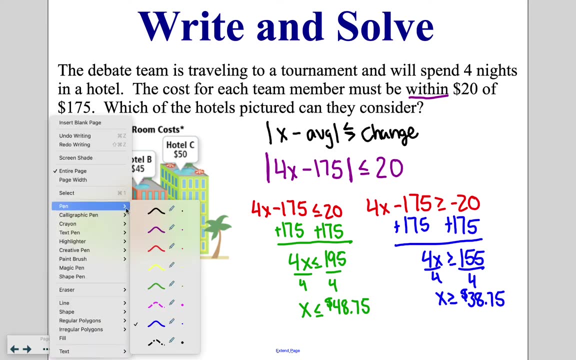 Dividing by four on both sides, I get X is greater than or equal to $38.75.. So what that means now is our answer has to be between $38.75 and $48.75.. So it has to be in between those two values. 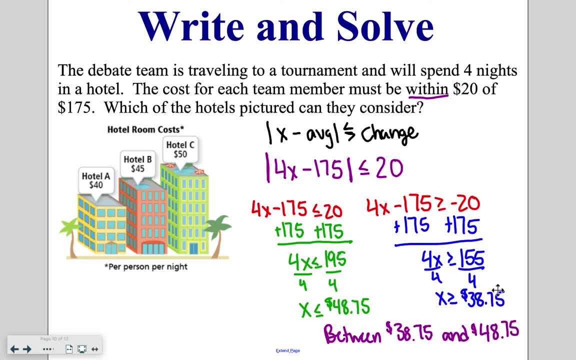 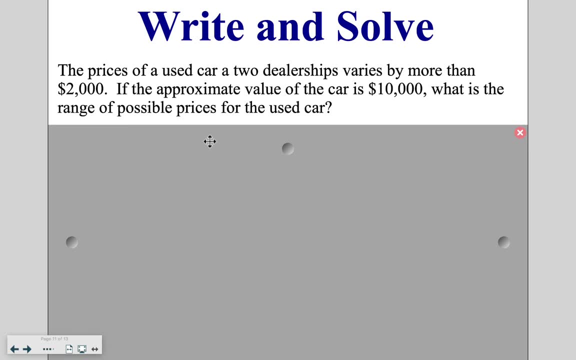 So if we go back to the original question of which hotels could they consider, the correct answers would be Hotel A and Hotel B. Hotel C is too expensive for their price range. Go ahead and try this one on your own. The first thing I want you to do, 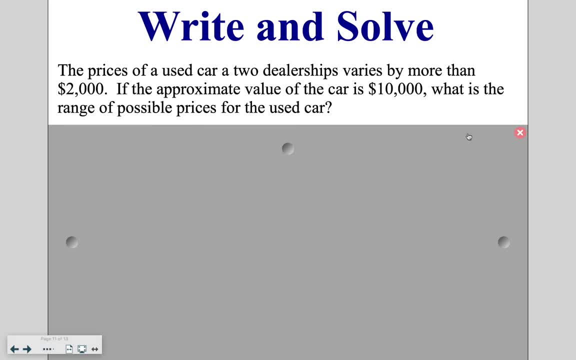 is just write the absolute value, inequality. So when you write your inequality, you get the absolute value of X minus 10,000, that's central cost for the price, And then it's going to be greater than $2,000.. The change is going to be more than $2,000.. 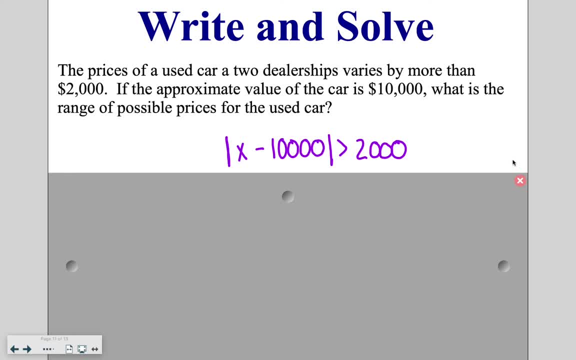 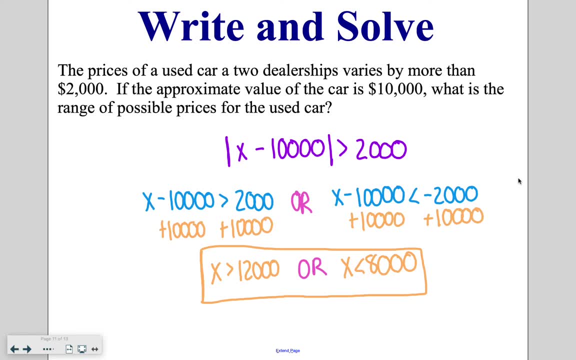 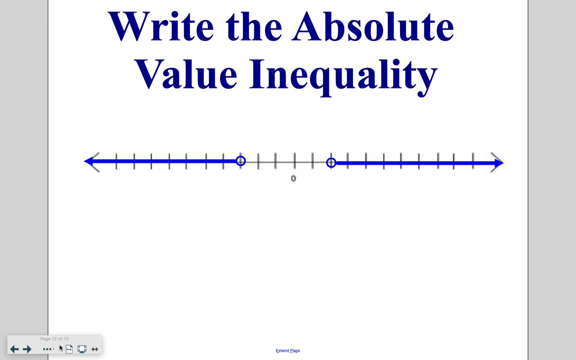 Now go ahead and solve case one and case two. When you solve, you find out that the price is either greater than $12,000 or less than $8,000.. The last piece here is writing the absolute value: inequalities. Once again, we are using that same general statement. 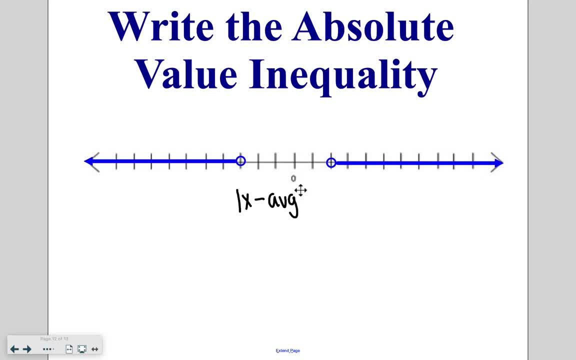 which is going to be X minus the average. So that central number is either going to be less than or greater than, and then the amount you're changing by. So, looking at this graph, we have an or statement and we know that or statements are going to be. 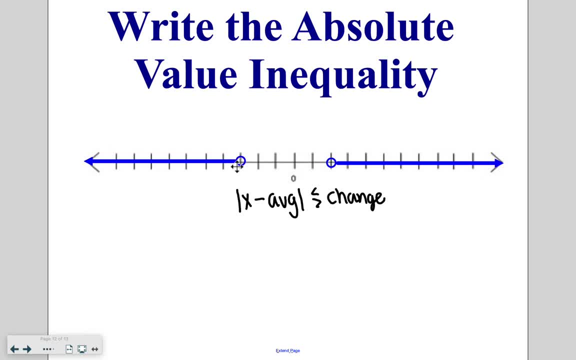 the greater than case. It's not greater than or equal to because our dots are not filled in. So now our job is to find that average value. If you remember from chapter two, in order to find average value on a graph, you take your low end point.